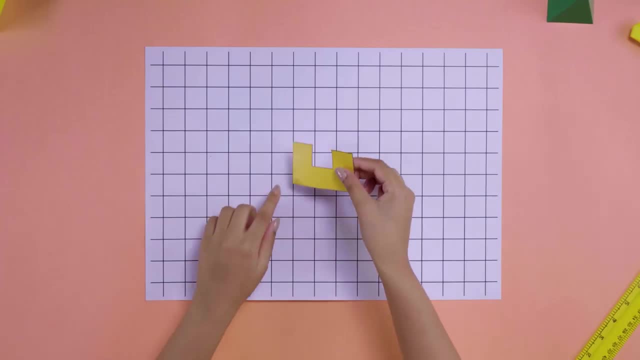 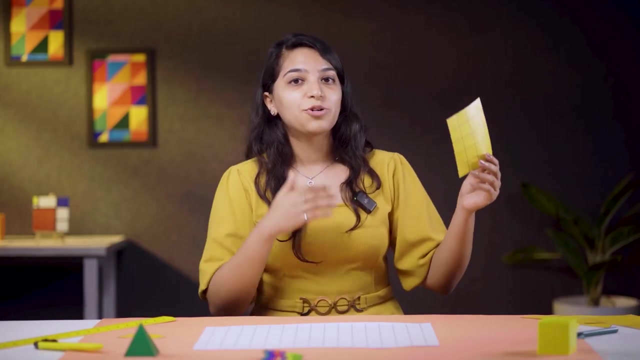 What's the area of any shape? It's the number of squares it covers on a flat surface. All these squares have side length of 1 inch. This shape covers 5 such squares, So its area is 5 square inches. It's easy to measure the area of any rectangle Like this. one has 5 squares in each. 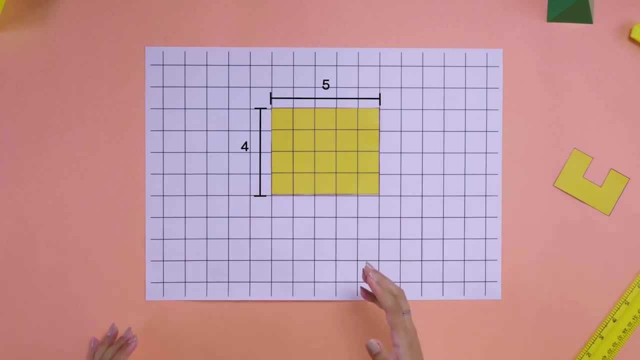 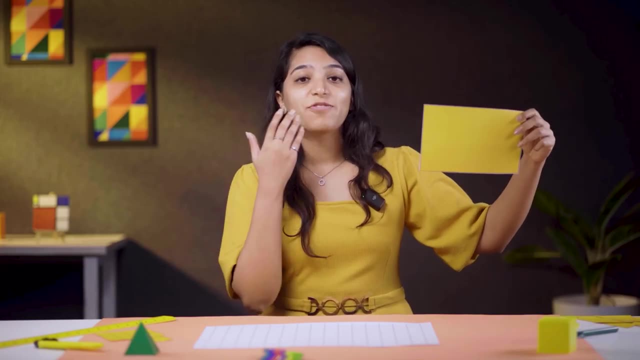 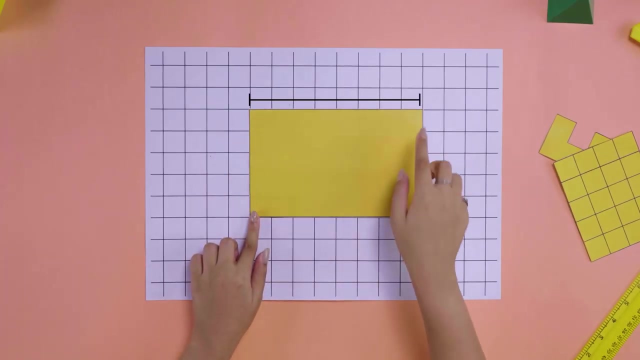 of its rows and 4 squares in each of its columns, So it covers 5 times 4, that is, 20 squares. This way, the area of any rectangle is simply the product of its two sides. For example, this side measures 8 inches and this side measures 5 inches, So its area is 8 times 5. 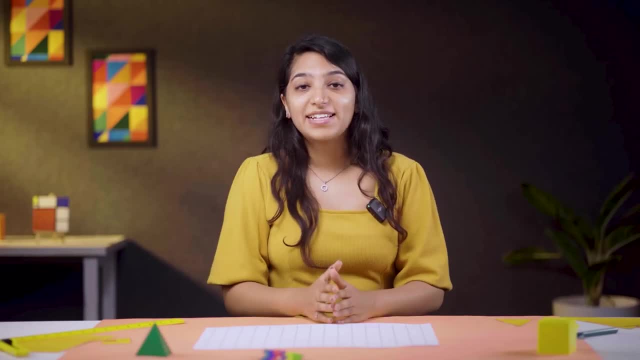 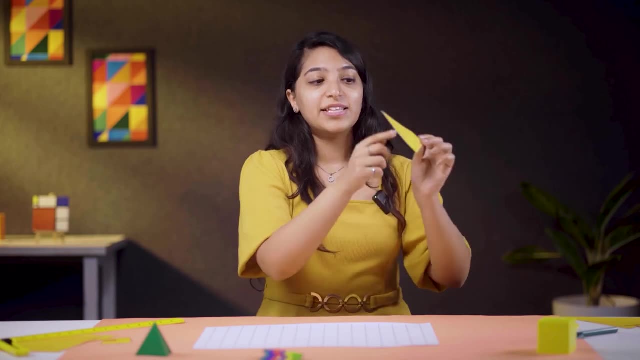 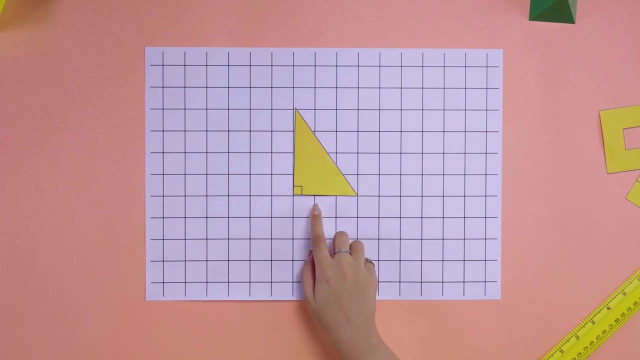 or 40 square inches. How do we find the area of any triangle? Let's start. Let's start with the simplest one: a right angle triangle. The two sides that make the right angle are called its base and height. To find its area, let's make a copy of this triangle and place it. 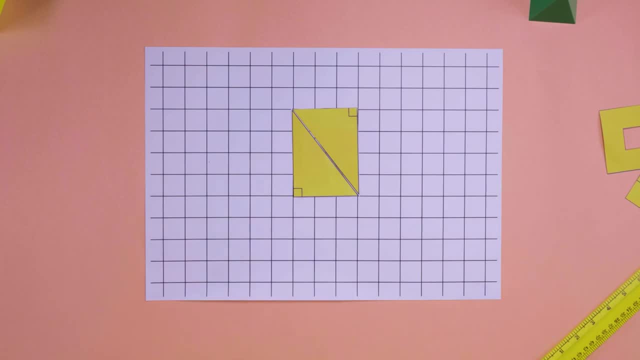 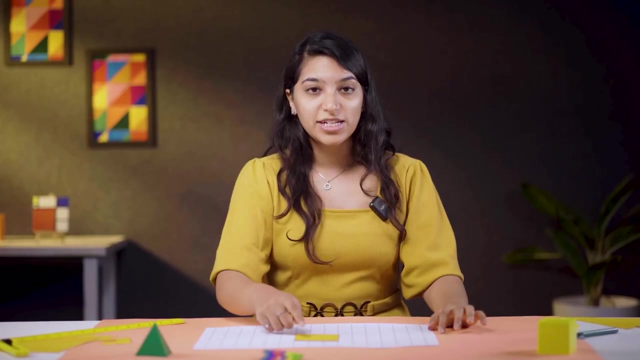 along the longer side. like this, This forms a rectangle with sides 3 and 4 inches. Now, what's area of a rectangle? The product of its adjacent sides, that is, 3 times 4, or 12 square inches. Since we use two such triangles, the area of this triangle must be half of 12, or 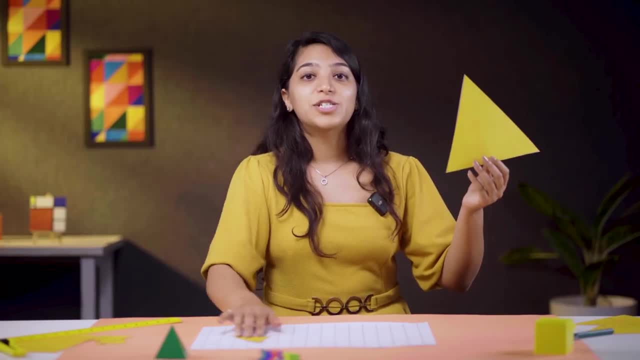 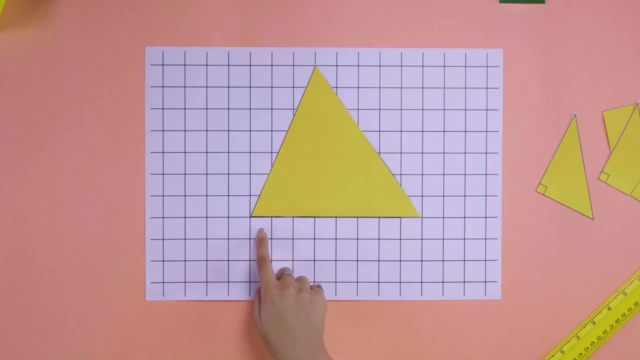 6 square inches. But what about a triangle which is not right angled? The trick is to break it into right triangles. For that, let's take this side as its base. Now, from the opposite corner, draw a line at right angles to its base. This forms two right triangles. 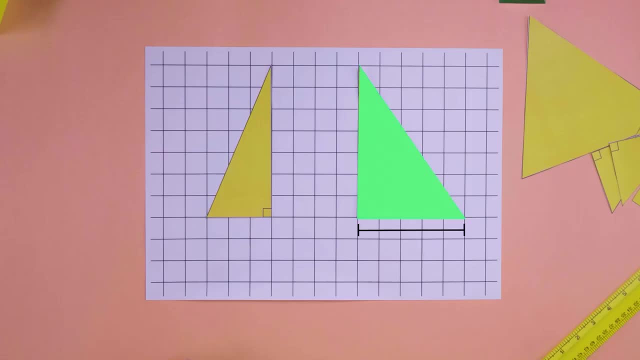 Now what's their area? The base of this one measures 5 inches and height measures 7 inches, So its area is half times 5 times 7.. Similarly, the base of this one is 3 inches, So its area is half times 3 times 7.. Let's add them up Now, we can factor out half times 7.. So we'll get the area. 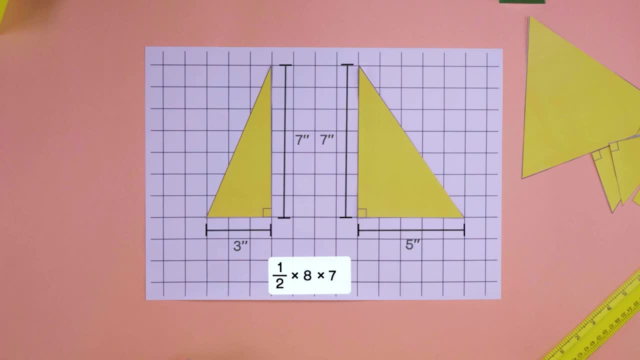 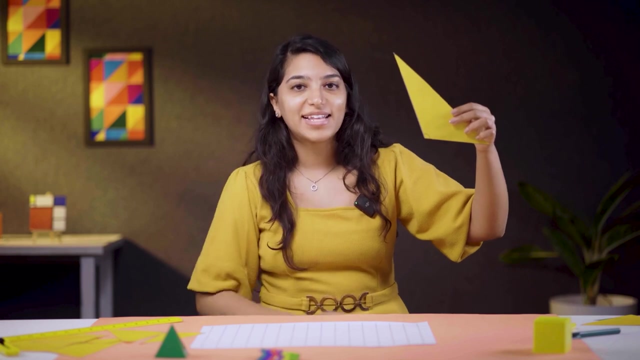 as half times 7 times 8.. And once again the area of our triangle turned out to be half times base times height, or 28 square inches. Now, how about this triangle with one angle bigger than 90 degrees? For that we will have to extend its base and then draw the. 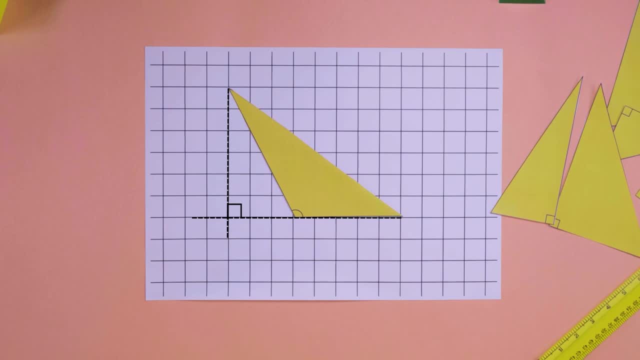 height from the opposite corner And once again we have two right triangles: This one and the bigger one. Subtracting the area of the right triangle, we get the area of the left triangle And once again we have two right triangles, This one and the bigger one Subtracting the area of. 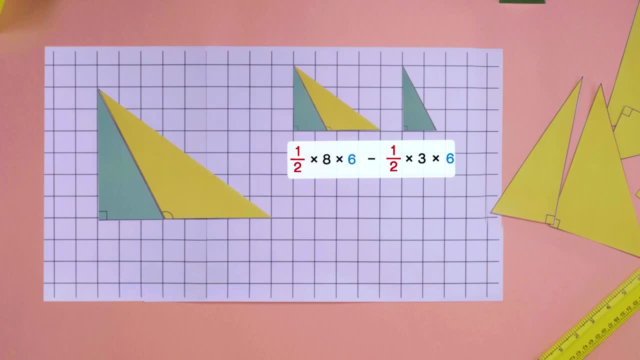 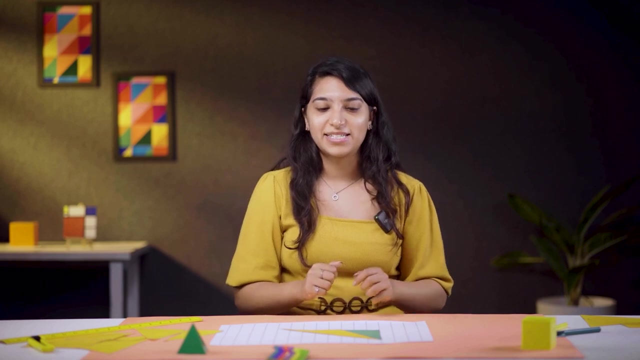 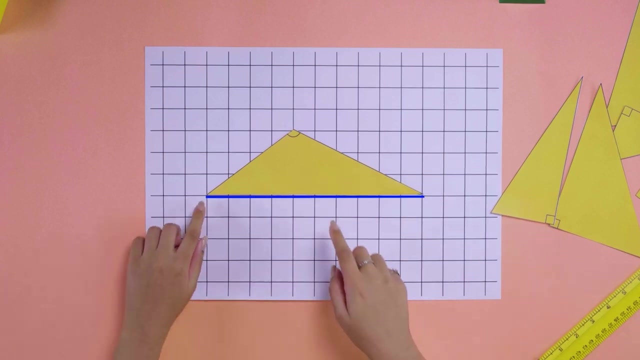 the smaller triangle from the bigger one. we'll get this And once again, the area of this triangle turns out to be half times base times height. In fact, we can take any side of the triangle as its base. Like for this triangle, we can take this side as its base. Now, the height: 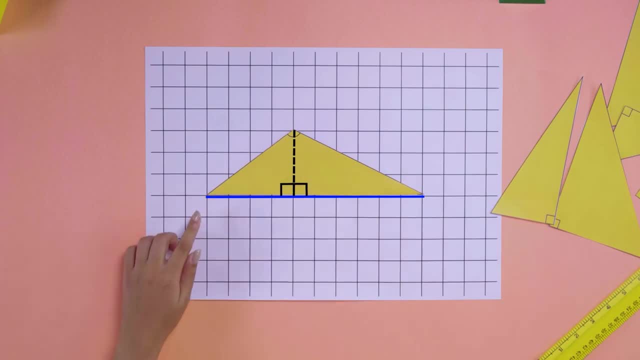 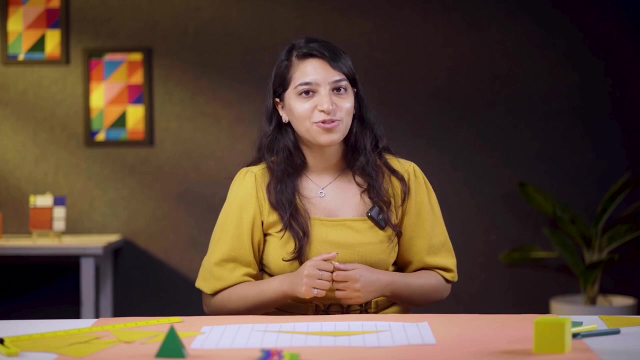 will be the line drawn to it at right angles from the opposite vertex. These two measure 10 inches and 3 inches, So its area is half of their product, or 15 square inches, Same as what we got from the other side. Now you know how to find the area of any triangle, Simply. 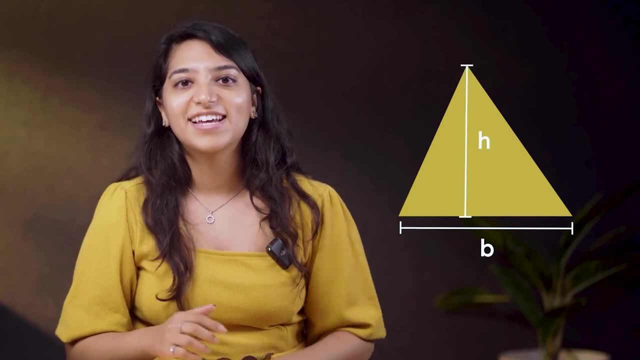 measure any one of its sides and the corresponding height. The area will be half times base times height. 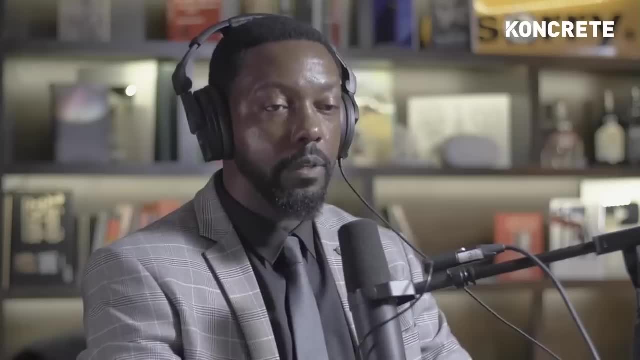 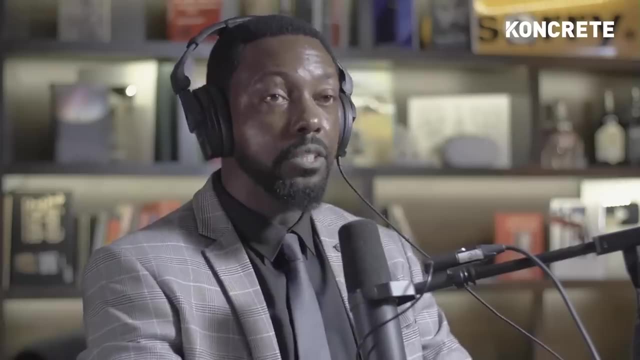 So I dug real deep into it and I got to the understanding that we're living in a multi-dimensional universe and there's at least 11 dimensions, otherwise the universe would collapse. Each dimension is a 90 degree angle right above the next one, compactified, so they're sitting right on top of us.